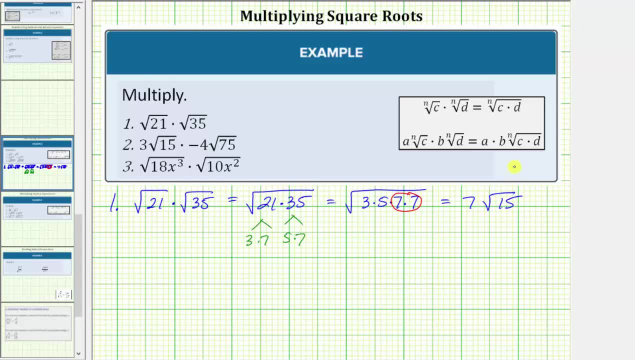 therefore this simplifies to seven square root fifteen. For number two, we have three square root fifteen times negative four square root seventy-five. Looking back at our notes, a times the answer root of c times b times the answer root of d equals a times b times the. 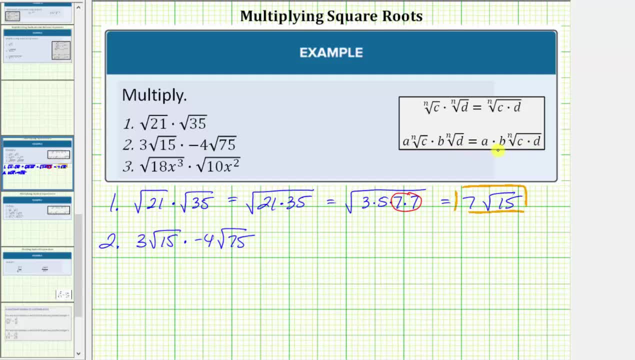 answer: root of c times d, Which means to find this product we multiply a and b outside the radical, and then multiply c and d, which are the radicands under the radical. So for number two this product is equal to three times. 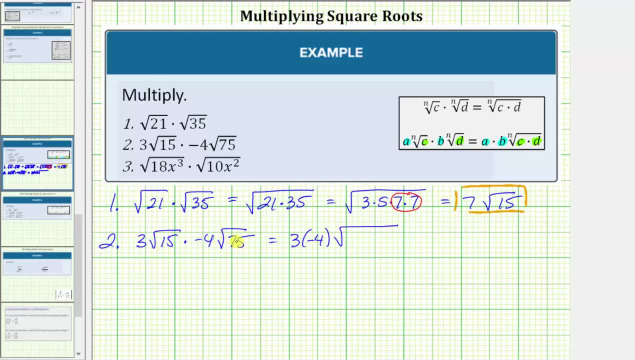 negative four times the square root of fifteen times seventy-five. Three times negative four is equal to negative twelve. and now let's determine the prime factorization of fifteen and seventy-five. Fifteen is equal to three times five. seventy-five is equal to three times twenty-five, and twenty-five is equal to five times five. 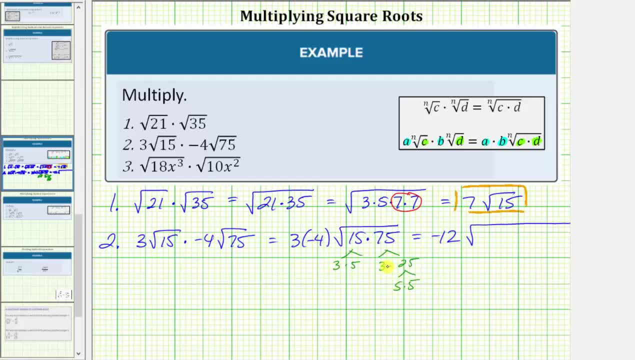 So the prime factorization of this product is three times three times five times five times five. And now we circle the perfect square factors of the radicand. Three times three is a perfect square, and so is five times five. Simplifying, we have negative twelve times the square root of three times three, or the square root of three. 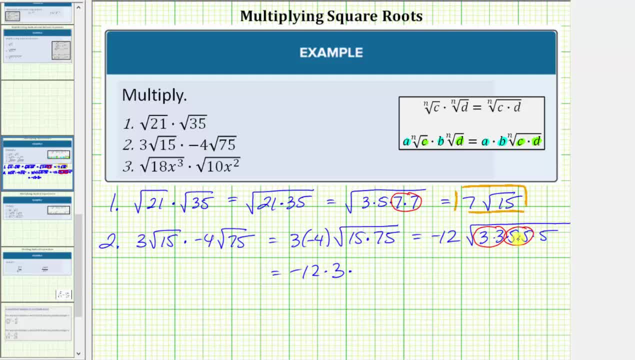 squared is one factor of three times the square root of five times five, or the square root of five squared is equal to one factor of five, and we still have the square root of five Negative twelve times three times five is equal to negative one hundred eighty. This 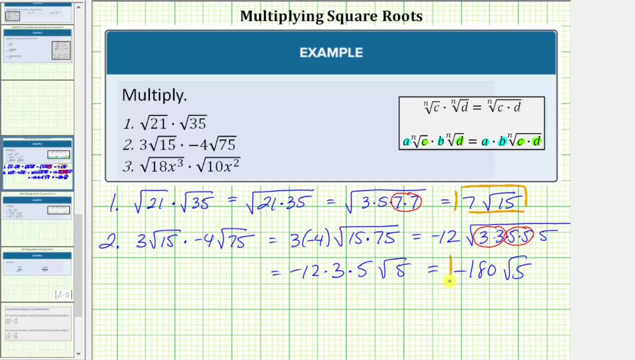 simplifies to negative one hundred eighty square root of five. And now for number three. we have the square root of eighteen, x to the third times the square root of ten x squared, This is equal to the square root of eighteen times ten times x raised to the power of three plus two, which gives us x to the fifth. 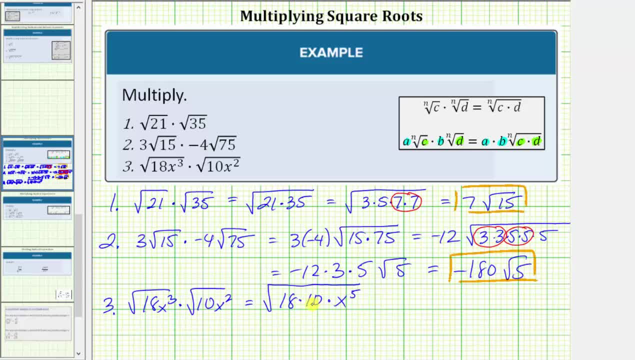 For the next step, we'll determine the prime factorization of eighteen and ten. Well, eighteen is equal to two times nine, nine is equal to three times three. ten is equal to two times five. So for the prime factorization, we have two factors of two, two factors of three and a factor of five. 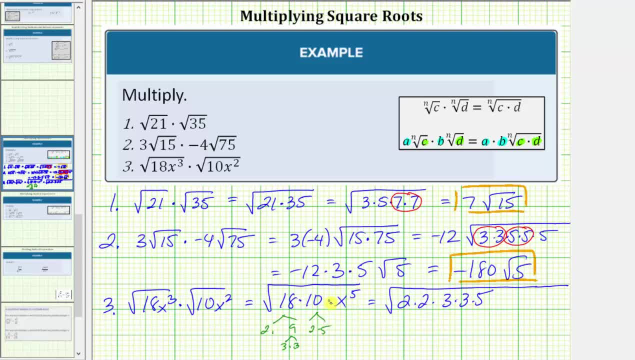 X to the fourth is the perfect square of x to the fifth. To show this, we'll write x to the fourth as x to the second, times x to the second, And we still have times. one more factor of x, And now we'll circle the perfect square. 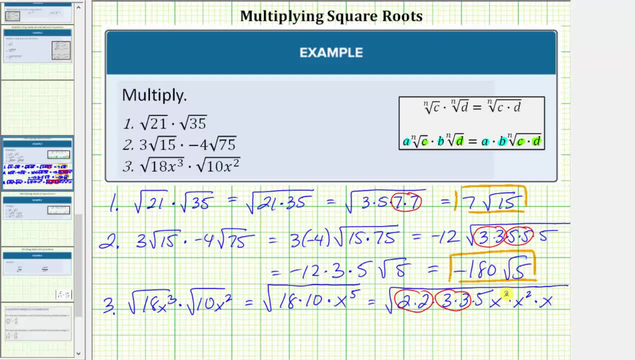 factors which are two times two, three times three and x squared times x squared. So, simplifying: the square root of two times two is equal to one factor of two. the square root of three times three is equal to one factor of three. 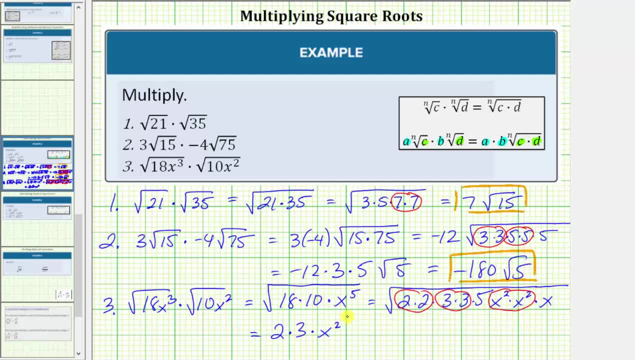 The square root of x squared times x squared is equal to one factor of x squared, and we're still left with the square root of five x. So the final result is six x squared times the square root of five x. And because the exponent on x is even, 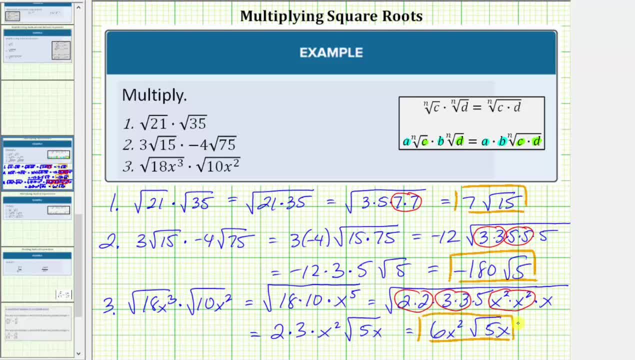 no absolute value is required. I hope you found this helpful. Thank you. 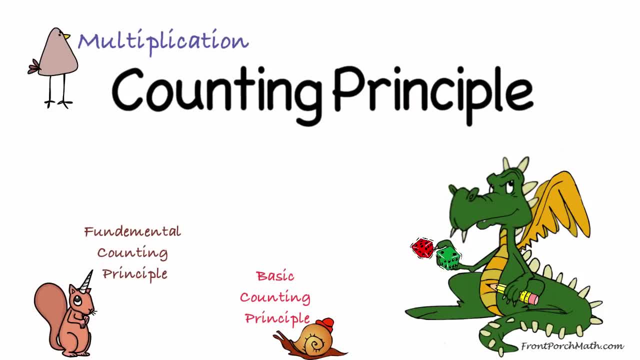 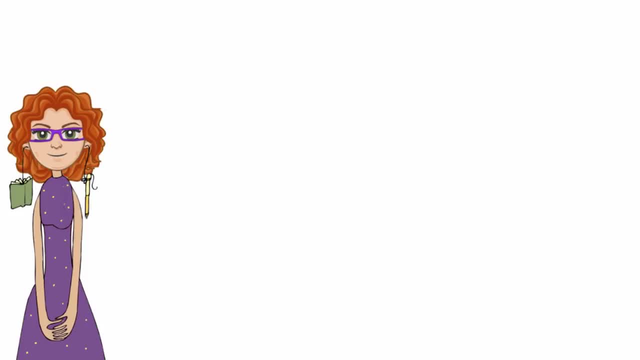 So today we're going to be learning about the counting principle. This is often used in probability and statistics to figure out how many possible options there are. So let's start with the situation that I bring my lunch to school every day. At home, I've got 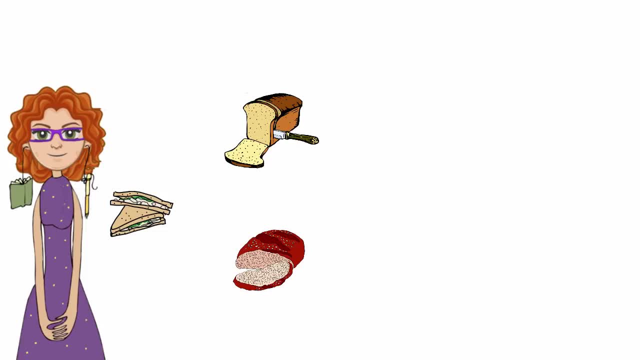 two types of bread: wheat bread and rye bread. I also have three types of fillings I like to use. I like tuna fish sandwiches, I like cheese sandwiches and I like peanut butter sandwiches. How many different combinations can I make so that I can have a different sandwich each day? 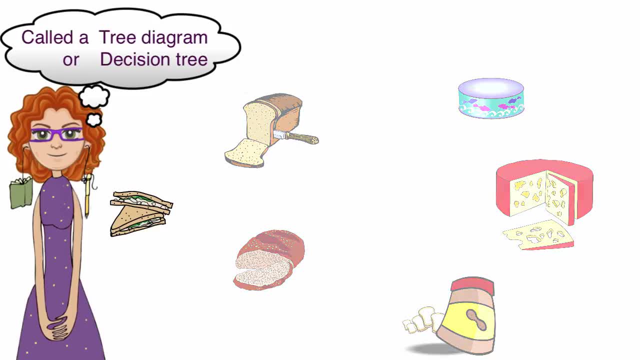 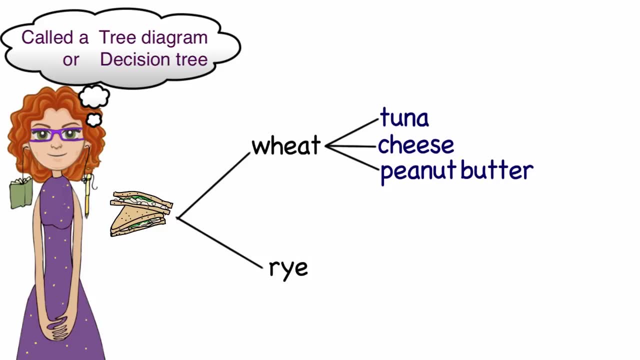 of the week. Well, one way to find that answer is to draw it out. I've got wheat and rye, and then for wheat I have the three options of tuna cheese or peanut butter, And for rye I have three options of tuna cheese and peanut butter, And we can see pretty quickly that we